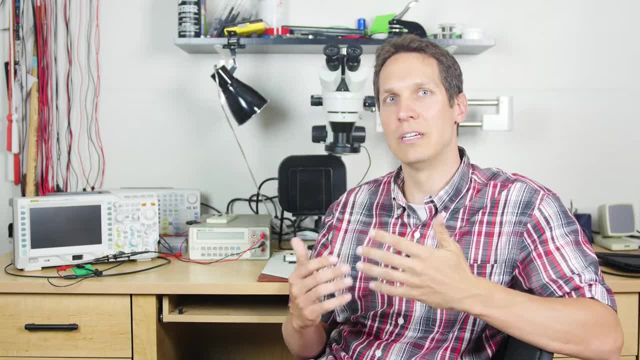 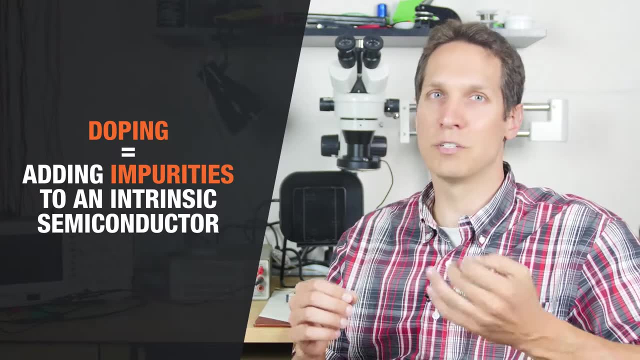 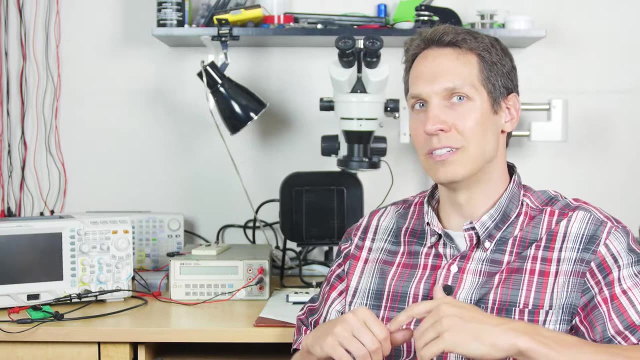 This is because of the limited number of free electrons and holes in it, but through a process known as doping, the conductivity of a semiconductor can be increased. Doping increases the number of current carriers by adding impurities with either more free electrons or free holes to the intrinsic semiconductor material. 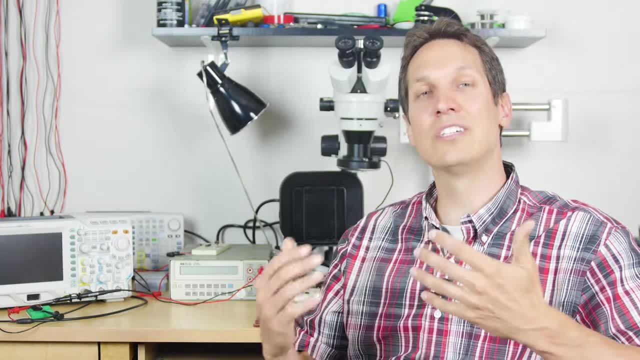 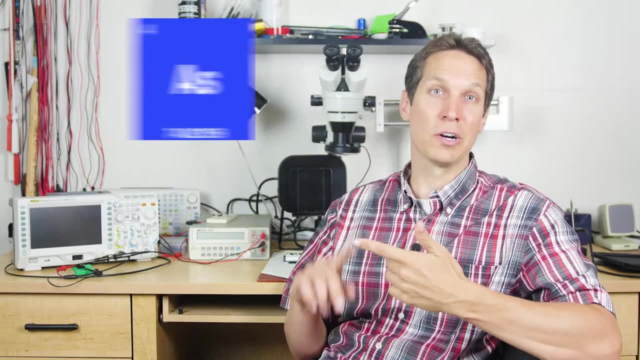 The number of free electrons and holes in the valence band is equal to the number of electrons in an intrinsic semiconductor material is increased in the doping process by adding pentavalent impurity atoms or atoms with five valence electrons, such as arsenic, phosphorus. 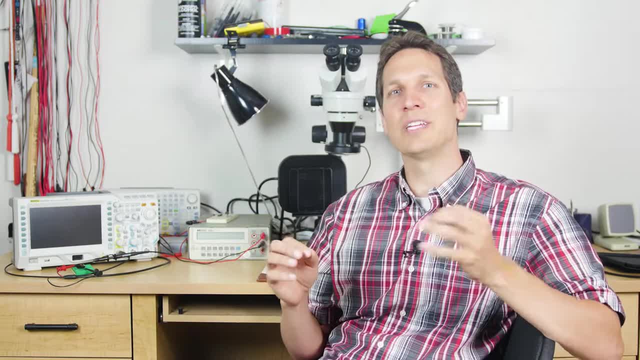 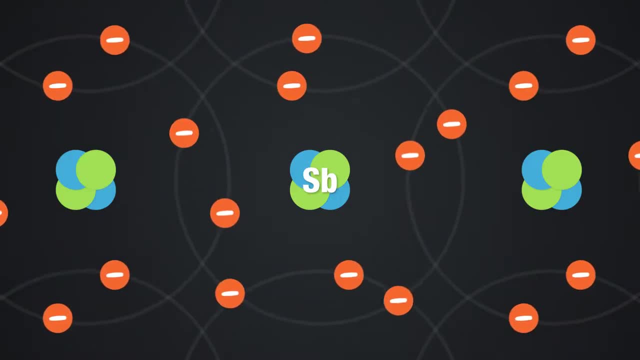 bismuth or antimony. To visualize this, let's examine an antimony atom covalently bonded with four adjacent silicon atoms. As we can see, only four valence electrons of the antimony atom are used to form covalent bonds with the silicon atoms, leaving an extra electron that becomes 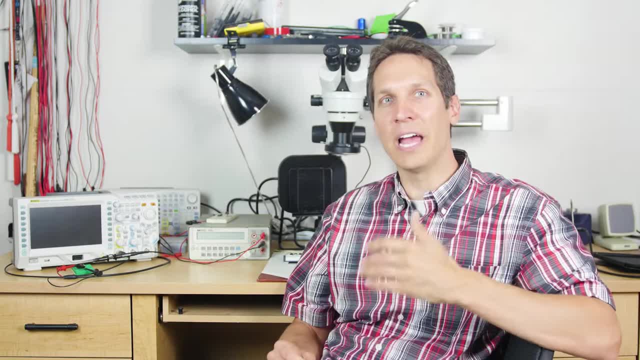 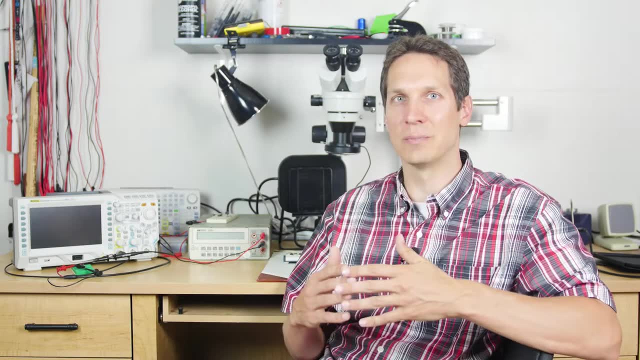 a free electron. So by adding pentavalent impurity atoms to an intrinsic semiconductor material, the number of free electrons can be increased, as well as the conductivity of the semiconductor material. Semiconductors doped with pentavalent atoms are n-type semiconductors, since the 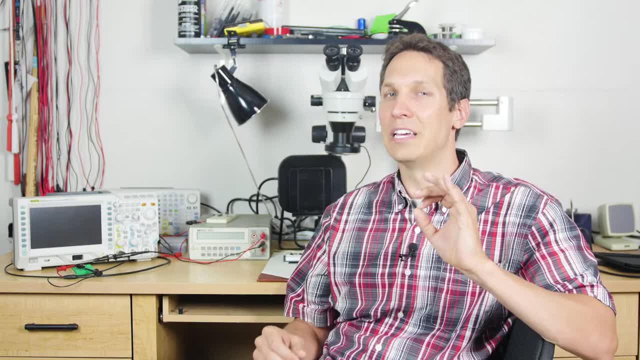 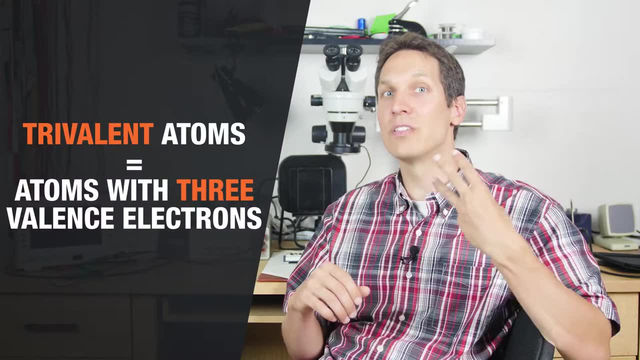 majority of its current carriers are electrons. In order for an intrinsic semiconductor material to have more holes, they are doped with trivalent impurity atoms. These are atoms with three valence electrons in their valence shell, like boron, arsenic, phosphorus, bismuth, bismuth, bismuth. 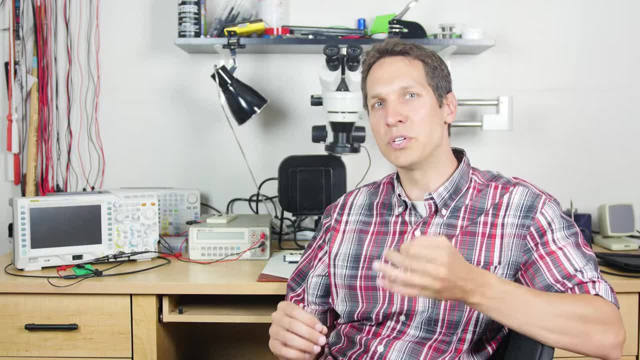 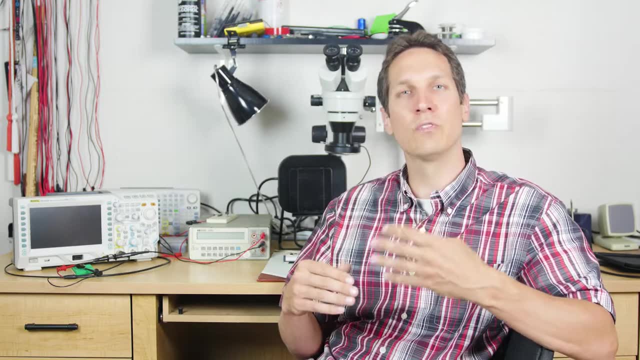 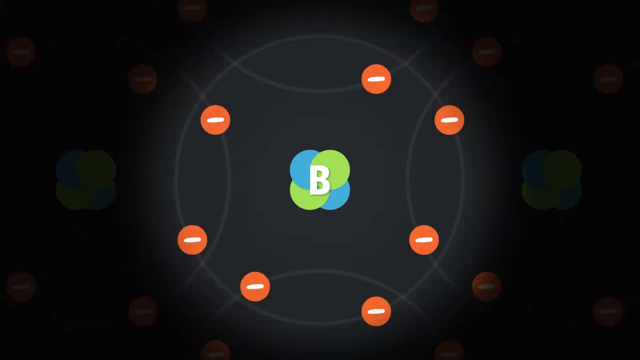 indium and gallium To understand how trivalent impurity atoms increase the number of holes in an intrinsic semiconductor material. let's see a boron atom form covalent bonds with four adjacent silicon atoms. In this case, when the boron covalently bonds with the four silicon atoms. 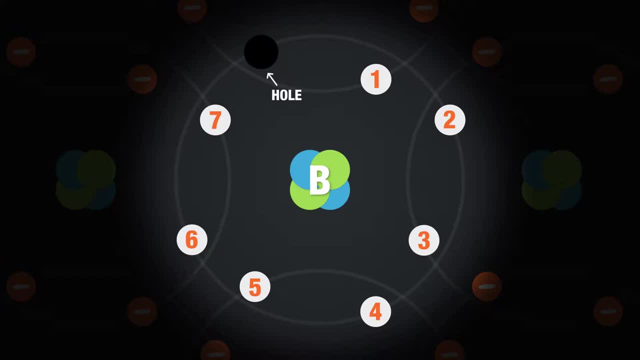 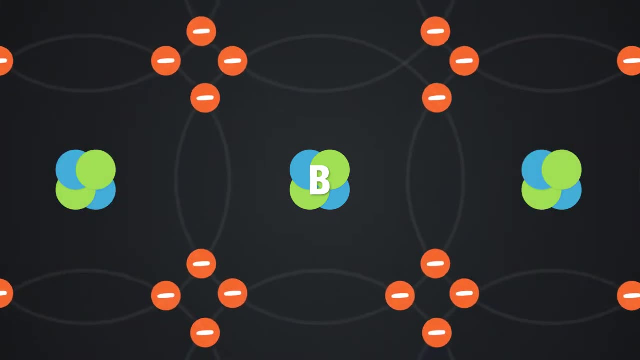 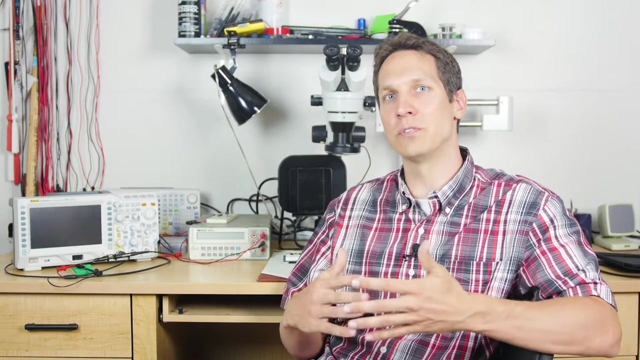 a hole is produced. This is because each of the four silicon atoms requires one electron from the boron atom, but it only has three valence electrons. In this case we can say that by adding the two silicon atoms to an intrinsic semiconductor material, it increases the number of holes and 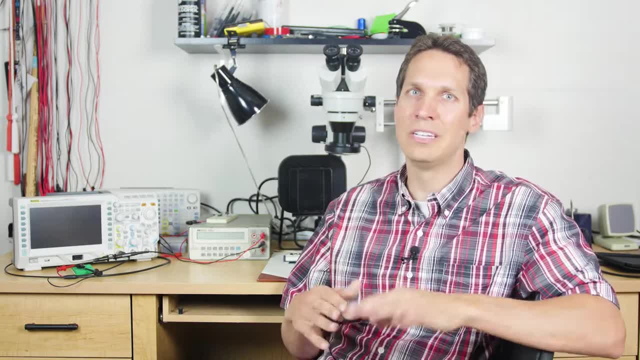 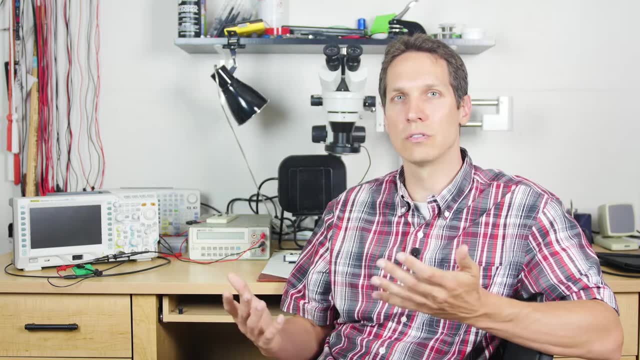 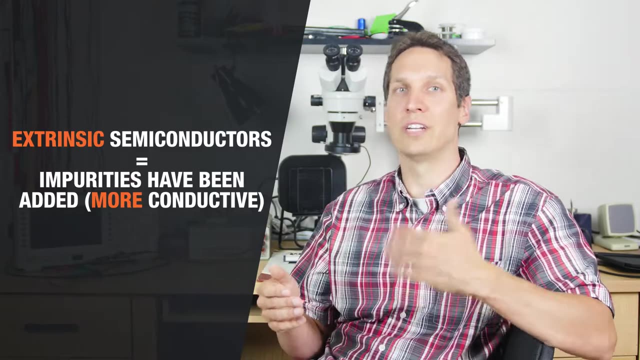 improves the conductivity of the semiconductor material. Semiconductors doped with trivalent atoms are p-type semiconductors, since the majority of its current carriers are holes. The doping process converts an intrinsic semiconductor material into extrinsic and produces either an n-type or p-type semiconductor material Combining the n-type and p-type.